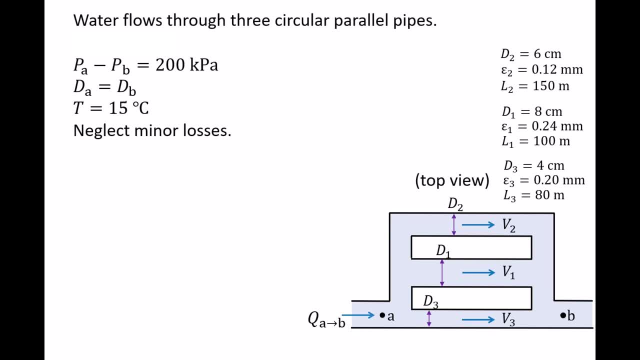 This is a reasonable assumption In many situations where there are very long runs of pipe. Based on the given information, we want to calculate the total volumetric flow rate flowing through the system Qab. Qab is found in the conservation of mass equation which, for a parallel pipe system, is Qab equals. 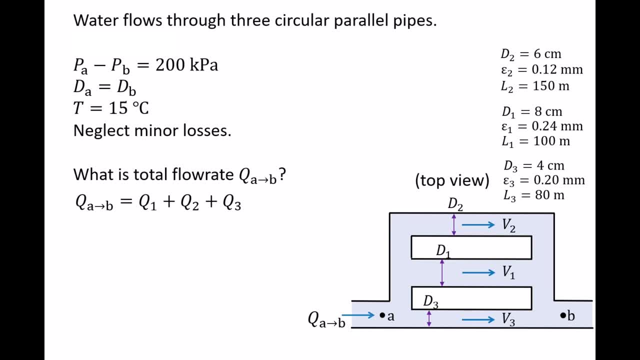 Q1 plus Q2 plus Q3.. The volumetric flow rate through each pipe is the flow speed V times the cross-sectional area, pi over 4 times d squared. So Qab is equal to V1 times pi over 4 d1 squared, plus V2 times pi over 4 d2 squared plus V3. 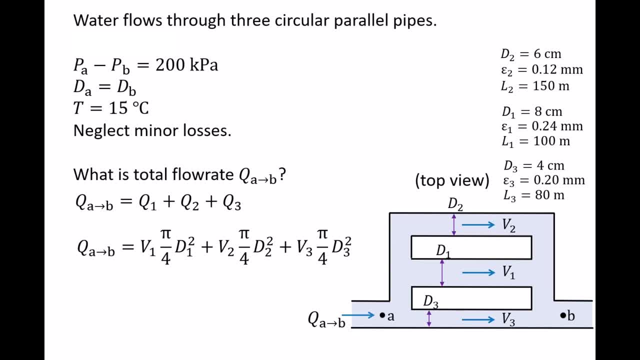 times pi over 4 d3 squared. At this point we know the diameters but not the speeds, so we will need to use conservation of energy to help us find V1,, V2, and V3.. We will apply the conservation of energy equation for each pipe individually. 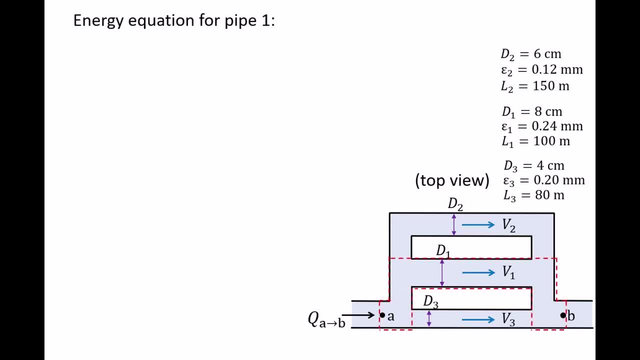 First we draw a control volume for the flow that goes through pipe 1.. The inlet is at point A and the outlet is at point B. The conservation of energy equation for this control volume is the pressure head plus velocity head plus elevation. head at outlet B is equal to the pressure head plus velocity. 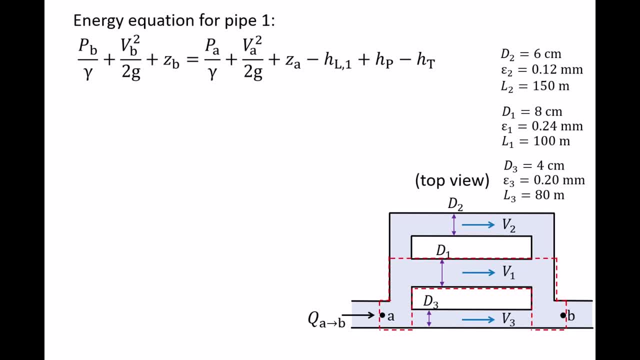 head plus elevation head at inlet A minus the head loss through pipe 1 plus the pump head minus the turbine head. Since we have steady flow and the pipe diameter at A and B are the same, the velocity at A and B are the same as well, and the velocity head terms cancel out. 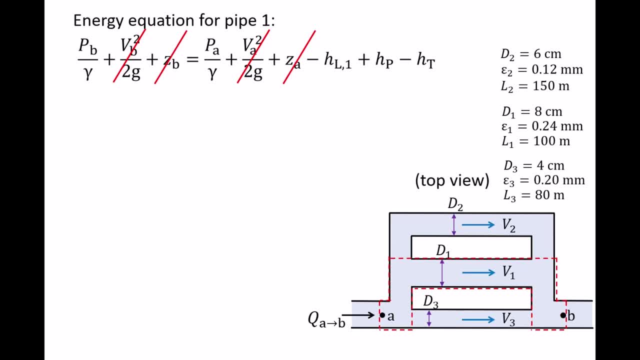 It was given that the inlet and outlet elevations are the same, so ZA and ZB cancel out as well. The pump head and turbine head are zero, since no pumps or turbines exist in the control volume. Rearranging the terms that survive, we find that the head loss through pipe 1, HL1, is 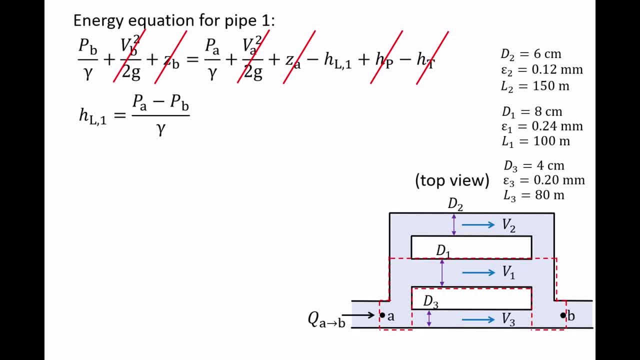 equal to the pressure difference PA minus PB, divided by the specific weight of water gamma. The pressure difference is 200,000 pascals and the specific weight of water at 15 degrees Celsius is approximately 9,800 newtons per cubic meter. 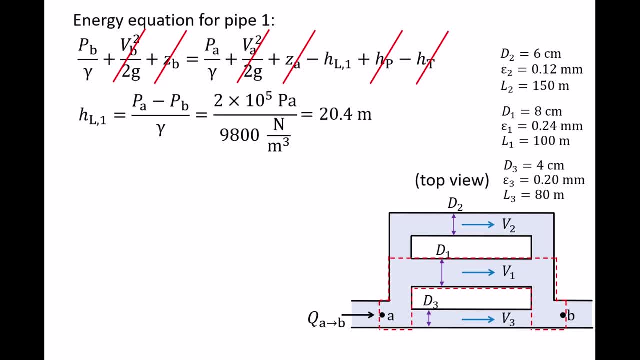 This gives us a head loss of 20.4 meters. In an earlier video, I showed you how to calculate the head loss through pipe 1, HL1, and pipe 1.. In an earlier video, we found that the head loss for parallel pipes that have the same 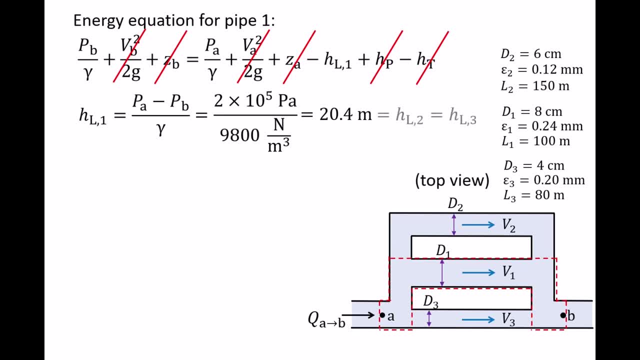 beginning and end conditions is the same, so the head loss through pipe 2 and pipe 3 also is 20.4 meters. Since the same equation applies to all three pipes, we will temporarily replace the subscript 1 in the energy equation with the subscript I, where I can be 1,, 2, or 3.. 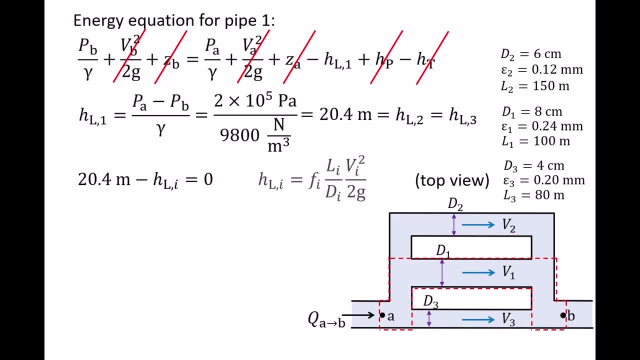 The major loss is the energy loss through pipe 1,, HL1, and pipe 3.. The major loss is the energy loss through pipe 2, HL1, and pipe 3.. The major loss through pipe I is calculated from the Darcy-Weisbach equation, which is: 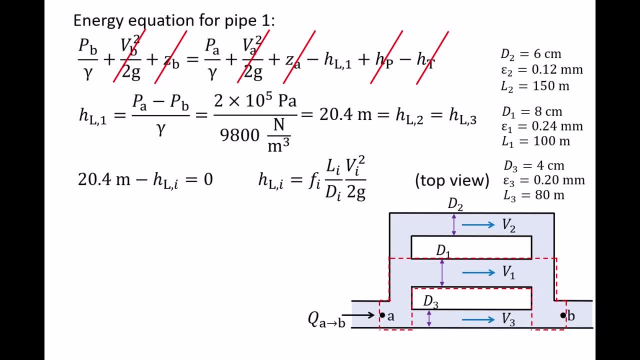 the friction factor Fi times pipe length, Li over pipe diameter, Di times speed, Vi squared divided by 2 times the gravitational acceleration g. If the flow is turbulent, the friction factor can be calculated from the Halland equation and is a function of the absolute roughness, epsilon i, pipe diameter, Di and Reynolds'. 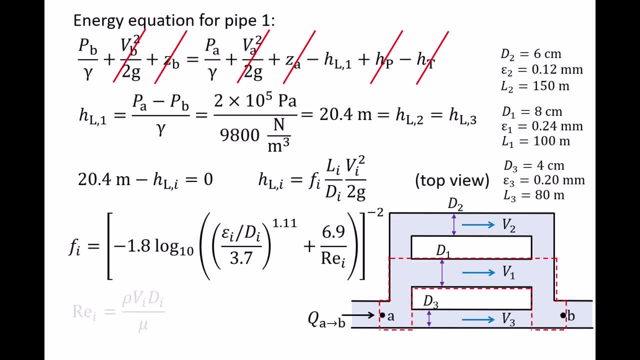 number Rei. The Reynolds' number for pipe I is fluid density: rho times flow speed, Vi times pipe diameter, Di, divided by the absolute viscosity, mu. There is no subscript I for density and viscosity because we assume those two quantities are constant throughout the flow. As mentioned earlier, the Halland equation should only be used for turbulent flows. 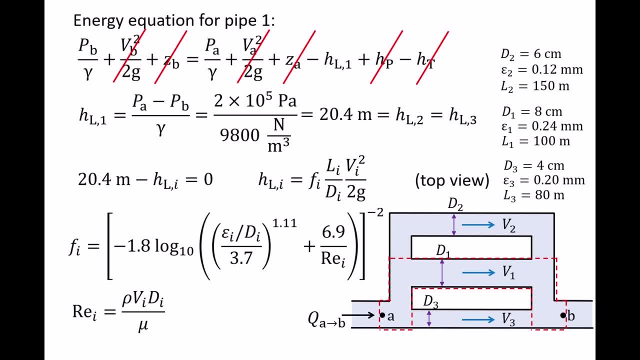 This occurs when the Reynolds' number is greater than 4.5.. At this point in the problem, we don't know the flow speed, so we don't know whether the Halland equation is valid. However, fluids like water and air usually experience turbulent flow conditions, so it's. 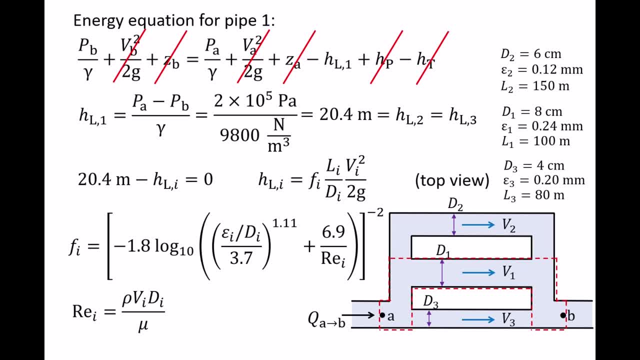 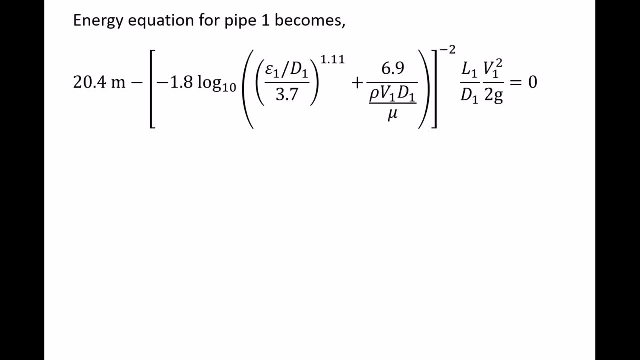 reasonable to start with an assumption of turbulent flow. After we obtain the value for the flow speed and can calculate the Reynolds' number, we will check whether the turbulent flow assumption was valid. Recap the Darcy-Weisbach and Halland equations into the energy equation and examine pipe 1. Note: 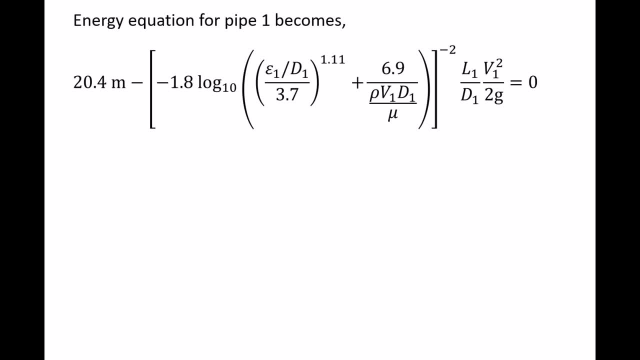 that the subscript i has been replaced by the number 1.. The diameter, absolute roughness and length of pipe 1 were already given. At 15 degrees Celsius, the density of water is 999 kilograms per cubic meter and the absolute viscosity is 1.14 times 10 to the minus 3. 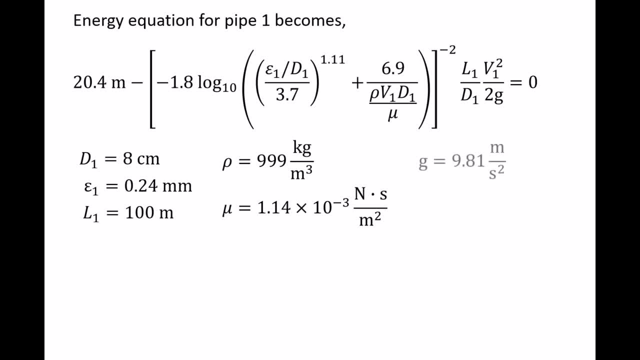 newton seconds per meter squared and the gravitational acceleration is 9.81 meters per second squared. This means the only unknown quantity in the equation is the speed v1.. Unfortunately, it's too difficult to solve this equation for v1 through algebraic manipulation. 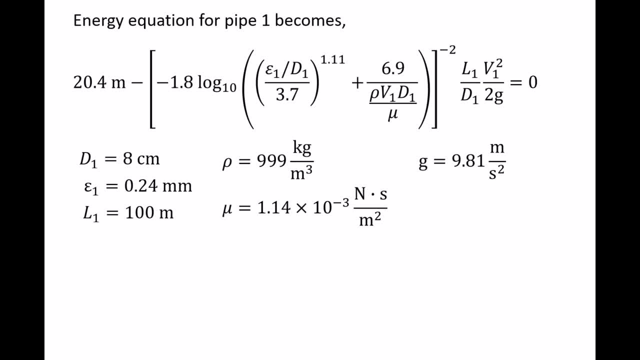 so we have three options. Notice that the right side of the equation is zero. This means we only need to find a value of 0.5.. We can then use the equation to solve the equation for v1.. The first option for solving this equation involves us guessing a value of v1 and then 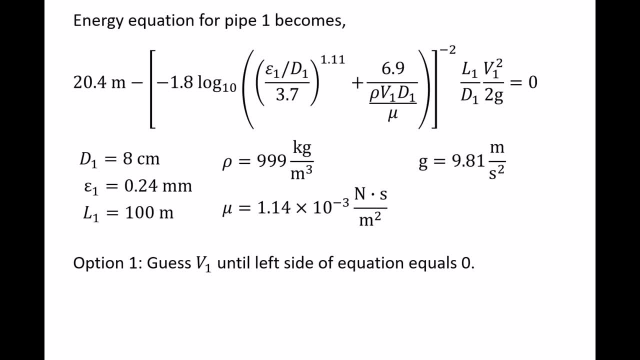 refining that guess until the left side of the equation is close enough to zero that we are satisfied. The second option is to use a numerical method to solve for v1 in a more systematic manner than just guessing. Common numerical methods that solve non-linear algebraic equations. 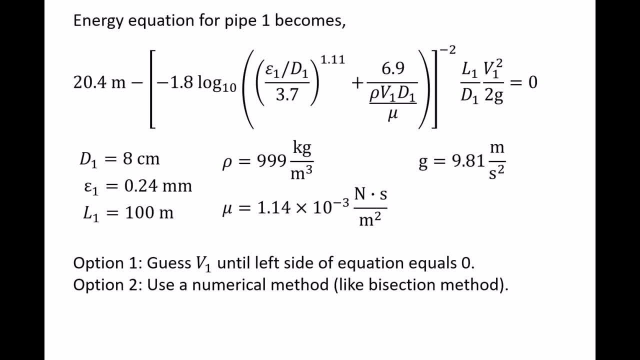 like the energy equation shown here are the bisection method, Newton-Raphson method and secant method. The third option is to use software that utilizes a numerical method to solve non-linear algebraic equations. For example, if you have access to MATLAB. 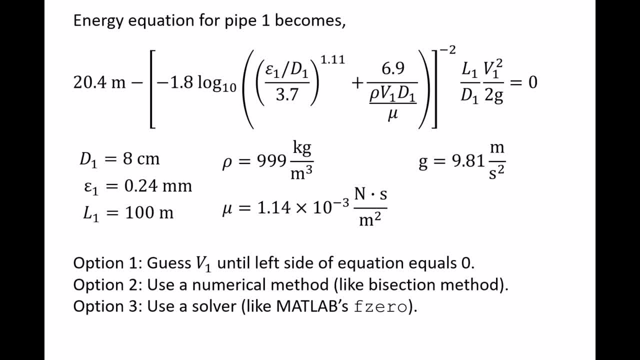 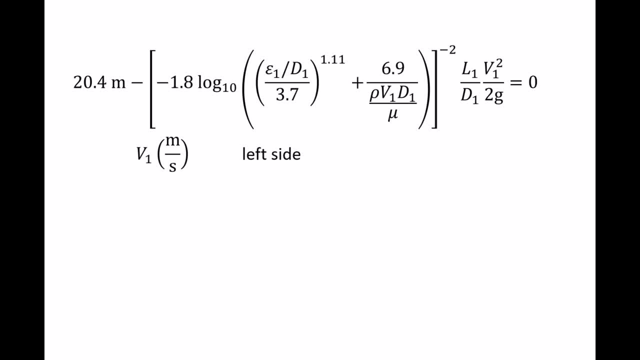 there's a built-in function called f0 that is fairly easy to use. Here's an example of how to find v1 using the first option. Let's start by guessing 10 meters per second for v1.. Plugging that value into the left side of the equation gives negative. 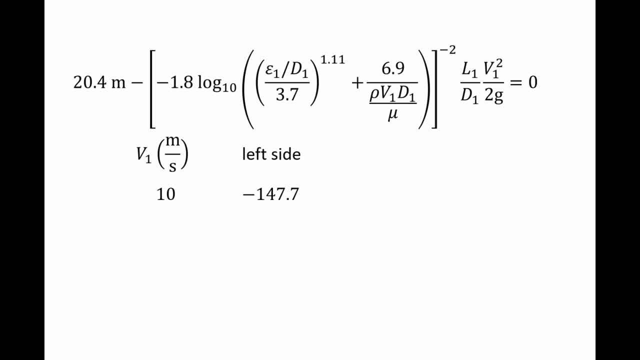 147.7,, which is not close to zero. So the actual value of v1 is probably not close to 10 meters per second. If we now try guessing 2 meters per second for v1,, the left side of the equation becomes smaller and positive: 13.50.. Since the sign has changed from negative to positive, 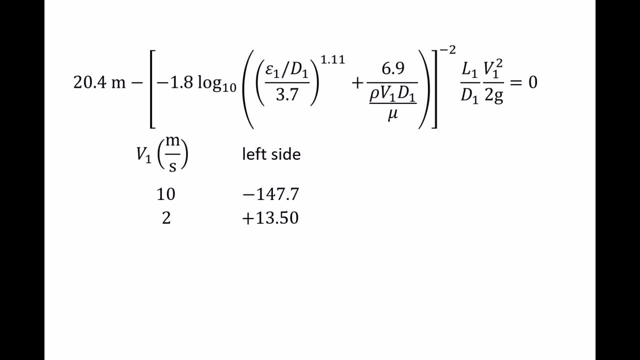 the value of v1 is between 2 meters per second and 10 meters per second, So let's try 5 meters per second. The left side of the equation becomes negative 21.91.. Since the sign has changed back to negative, we have overshot the actual value of v1.. So let's try a speed between. 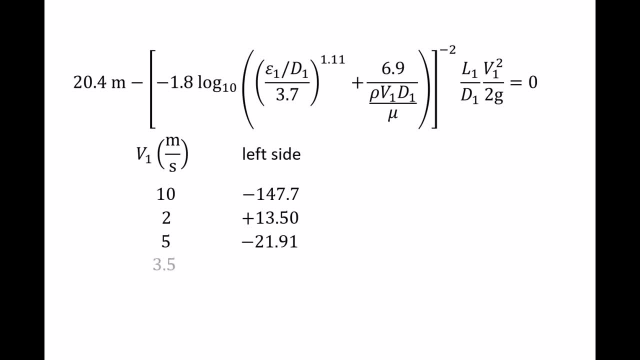 2 meters per second and 5 meters per second, like 3.5 meters per second. Now the left side of the equation has become much smaller in magnitude: negative 0.4456.. This means v1 likely is pretty close to 3.5 meters per second. We continue this process until v1 is equal to 3.462, which makes 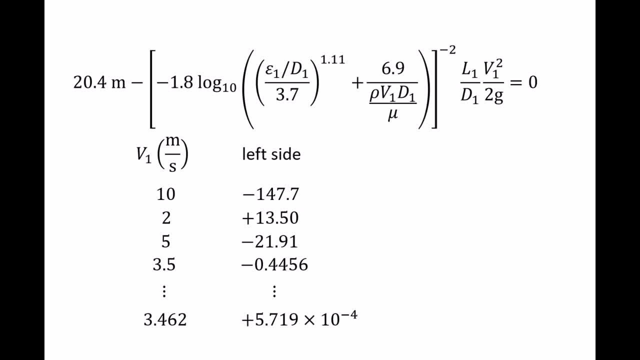 the left side of the equation, equal to 5.719 times 10, to the minus 4.. We could continue to refine our estimate of v1,, but since we don't know the actual value of v1, let's try 5.719 times 10 to. the minus 4.. We could continue to refine our estimate of v1,, but since we don't know the actual value of v1, let's try: 5.719 times 10 to the minus 4.. We could continue to refine our estimate of. 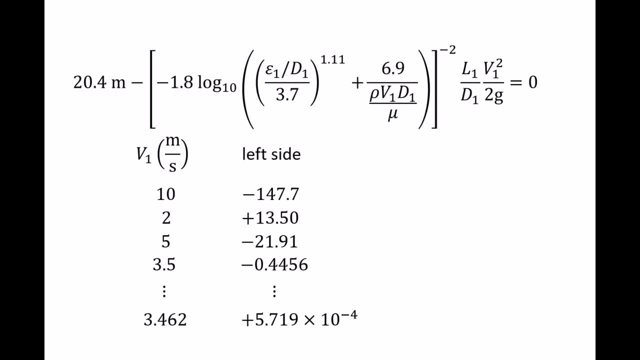 v1, but since we don't know the actual value of v1, let's try: 5.719 times 10 to the minus 4.. We likely don't know the values of the other variables, like pipe diameter and roughness to a. 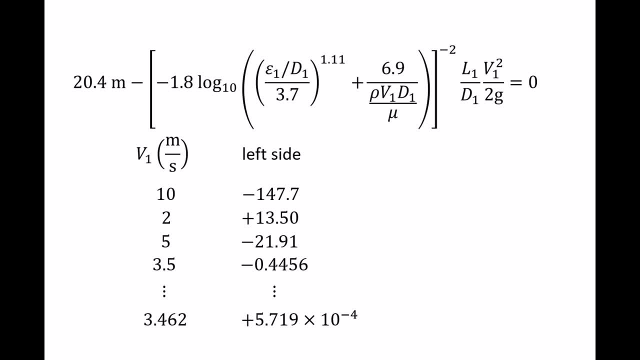 high level of accuracy and the Halland equation already has significant error built into it. finding v1 to 4 digits of accuracy is more than enough. At this point we should calculate the Reynolds number to verify the turbulent assumption was valid If the Reynolds number is above 4000,. 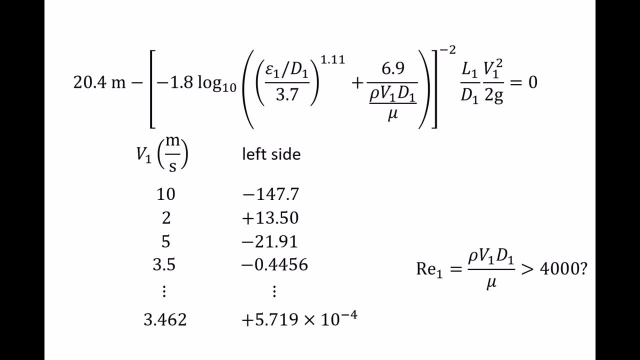 our value of v1 is good. If the Reynolds number was below 4000, you can try using the head loss expression for laminar flows, which was presented in a prior video. On your own you can verify. the Reynolds number is close to 240,000, which means we have found 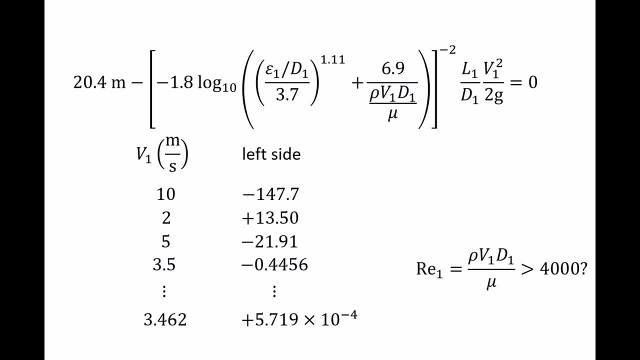 a valid value of v1.. Now that we have found a value for v1, we can calculate q1.. This process can be repeated to find v2 and v3 by replacing all the 1 subscripts with either 2 or 3.. 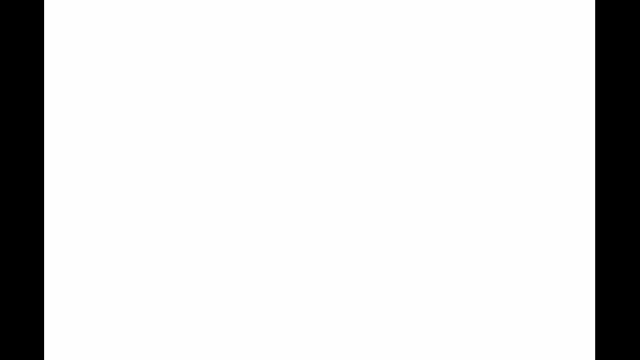 Now we're going to talk about a way to solve this problem quickly using the third option that was mentioned earlier. We will use the f0 function in MATLAB, One of the great advantages of using MATLAB- or any other software package- over the trial and error method that was just performed. 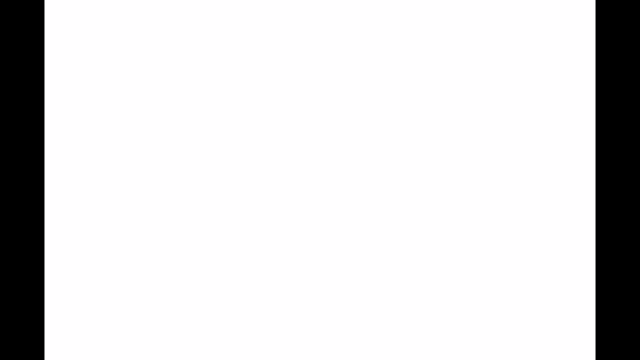 is that once you input the commands into MATLAB, it takes MATLAB almost no time at all to calculate the speed At the command line. in MATLAB, which is indicated by the double greater than symbols, we assign values for the known quantities of density, absolute viscosity, gravitational acceleration, length, diameter. 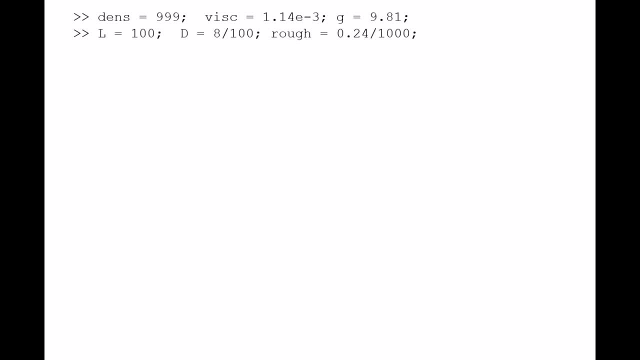 and absolute roughness, making sure that all the lengths are in meters. Next, we can create an anonymous function in the following manner: We need a name for the function, which is called the function handle, and I'm going to name this function energy, since it is the energy equation. The function energy equals at v and then the 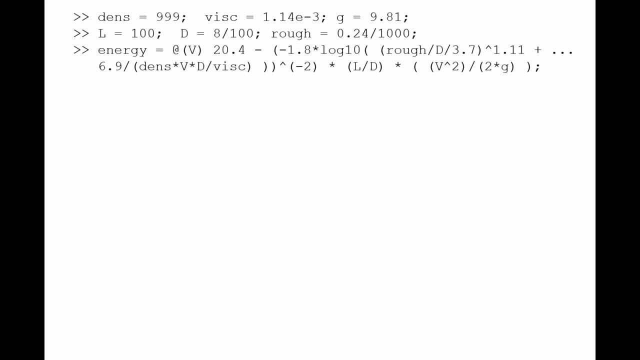 expression for the function handle is v. This function is called the function function, and the function is written in the upper right corner of the graph. MATLAB will now give an … equation that is called the f0 function, which is a function called the f0 function. after the energy equation is written, MATLAB will treat v as the quantity to be solved for, and it will treat all other variables, like density, viscosity and so on, as constants whose values are defined earlier in the code. The three dots in the middle of the equation simply indicate: 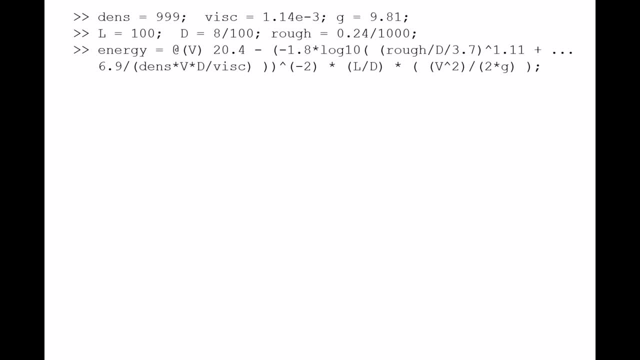 to MATLAB that the equation continues onto the next line. Now we can use the f0 function by writing: v1 equals f0, begin parenthesis, energy comma v2.. Now we can use the f0 function by writing: v1 equals f0, begin parenthesis, energy comma v2.. 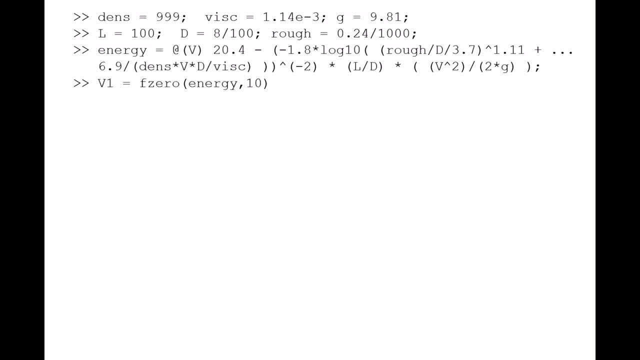 The first argument in F0 is the function handle, energy, and the second argument in the function, the number 10,, is our initial guess for the solution for the speed. It's okay to be wrong about the initial guess. MATLAB just needs an initial value to start its numerical method. 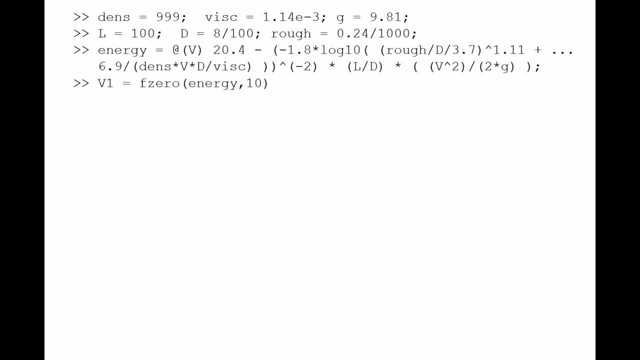 When F0 is finished, it will store the resulting value in the variable v1.. After hitting the enter key, F0 quickly returns 3.4620 and assigns this value to v1.. This is the value for v1 that will make the energy equation approximately zero.